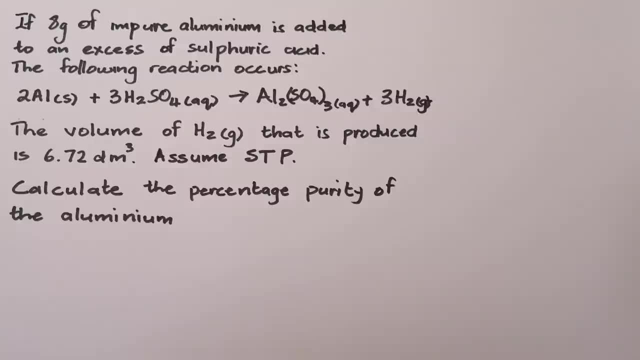 of a background of how we normally- You know, just you know- calculate percentage purity. So, essentially, I want you to imagine you've got this sample of, you know, aluminium. you know, in this case, aluminium. So, essentially, 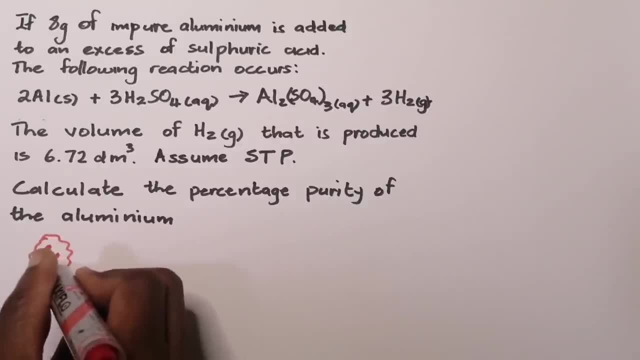 there are some impurities there. So, in actual sense, in the actual sense you can use, You can use the entire eight grams and say: well, I can calculate number of moles and therefore find out the you know number of moles from that mass. okay, Why is that? Because not all of those. 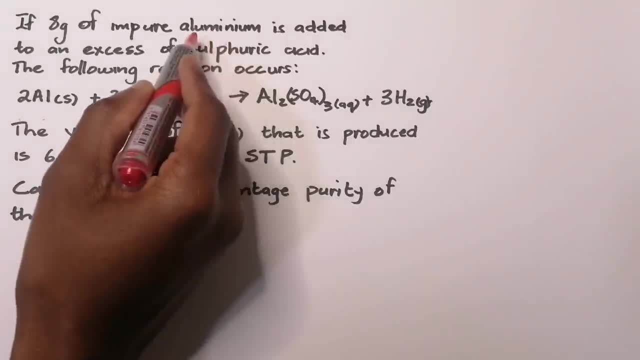 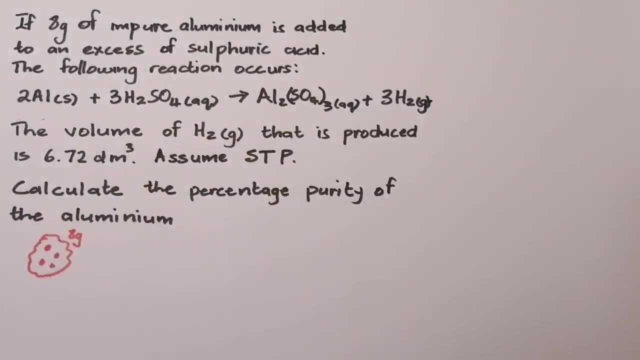 eight grams of aluminium. all right, or rather, not all of that eight grams is actually made out of aluminium, okay. So yes, truthfully, the aluminium is going to react with the sulphuric acid, the actual aluminium. So from that eight grams, remember. 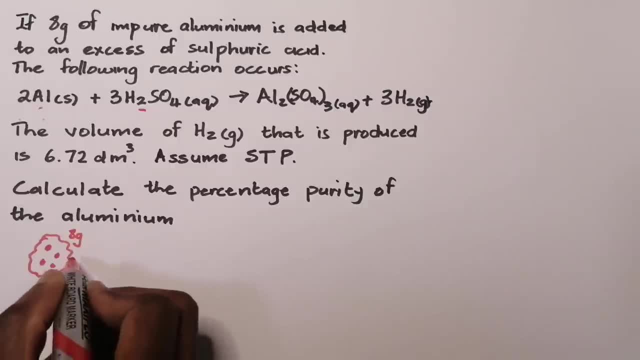 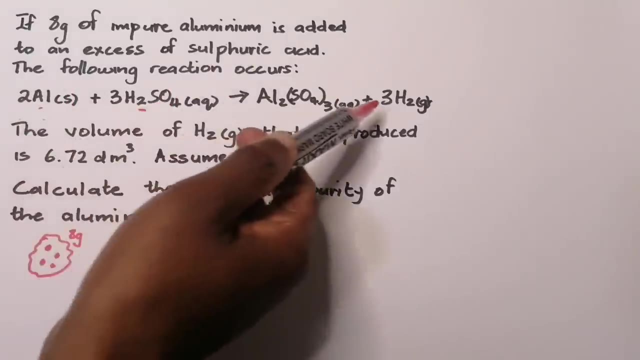 that I don't have the actual amount of the aluminium that's going to be there. However, I want you to think about it. So reaction between aluminium, the reaction between aluminium and sulphuric acid, would actually produce those products, Whatever impurities are there. 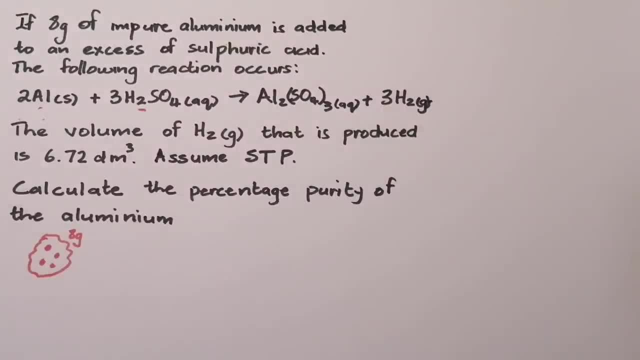 they cannot produce hydrogen, okay. So what I'm trying to say is, in these questions, what they do is they will probably give you an amount of the impure substance. okay, Of course, our assumption is that, or rather they told us that sulphuric acid is in excess. Now, the moment they tell us, 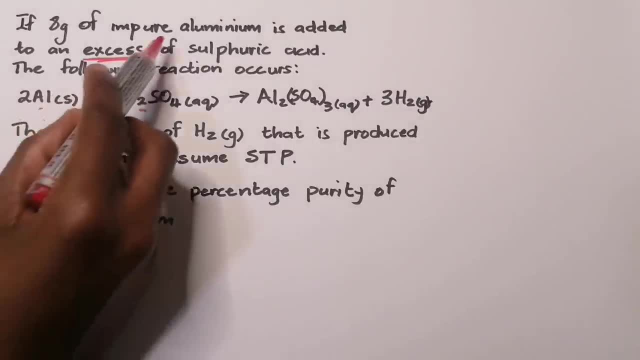 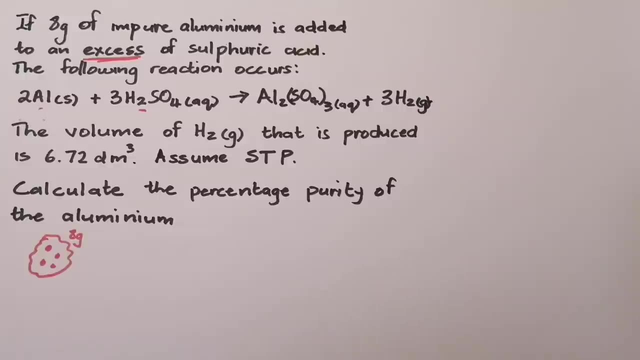 that sulphuric acid is in excess. it simply means that aluminium will be the limiting reagent. Please remember that, ladies and gentlemen. So that's the assumption. So the assumption is that aluminium will be the limiting reagent. Okay, Right. So of these eight grams, some of them are actually something else. Okay, Call it. 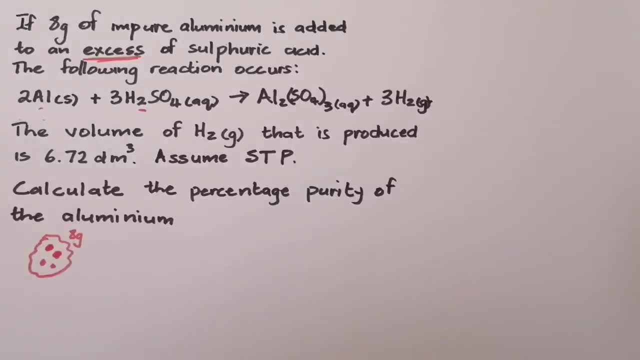 whatever, Okay, Right. So in this case, we simply want to find out how much of this eight gram is actually aluminium. All right, So I want you to stay with me And as we do this example together, okay, Right. So I'm simply going to say: 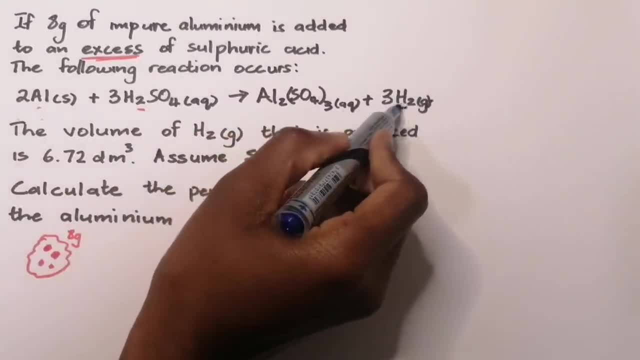 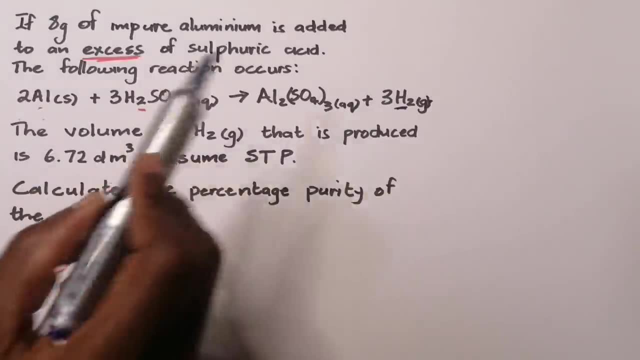 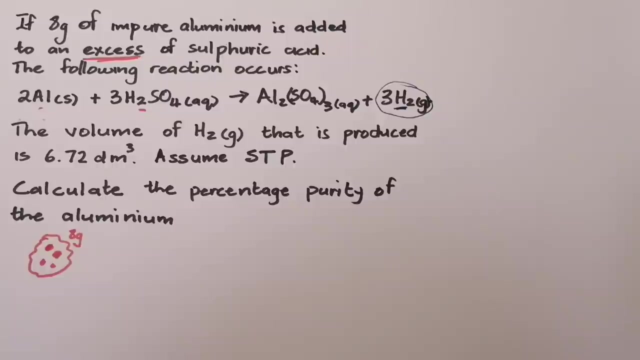 ideally, I'm going to get a hydrogen. And where does the hydrogen come from? It comes from the actual pure aluminium. So is it possible for me to find out the number of moles of hydrogen that I produce and, as a result, work my way back to then determine the moles of aluminium? Of course, 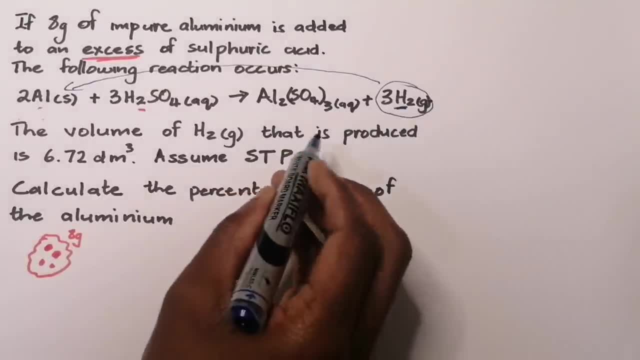 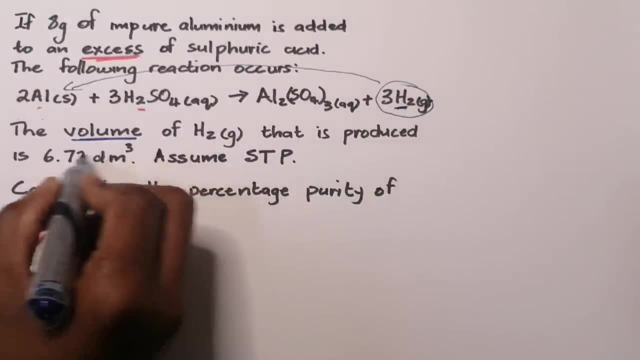 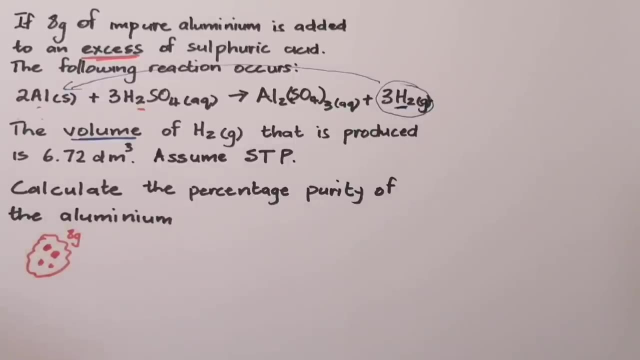 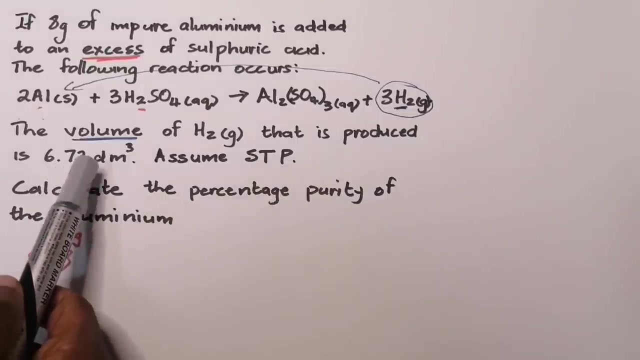 that's possible, right? So let's start right there. So I'm thinking this is a full time task, So I'm going to go back here and I'm going to come to the thing and I'm going to indicate to the 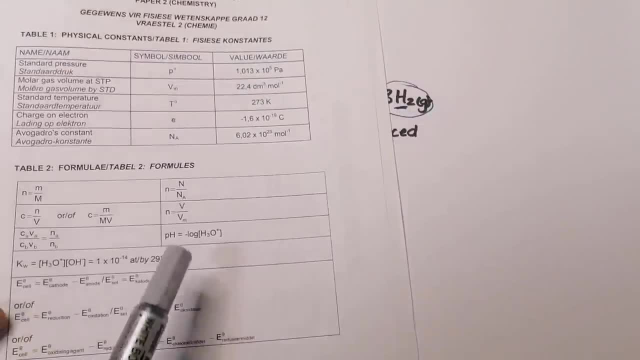 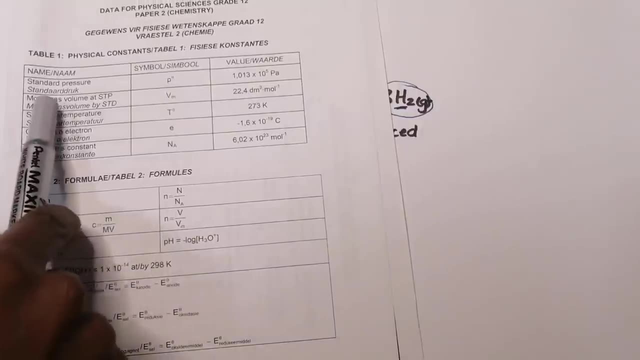 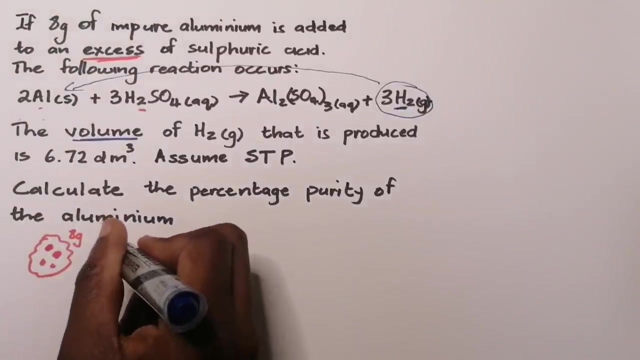 to convert it to moles and remember the formula to do that. that's number of moles, it's volume divided by the molar volume. and remember they told us it's at stp. so we know the molar volume at stp is actually 22.4, right? so now we know that the number of moles, remember this- is the number of. 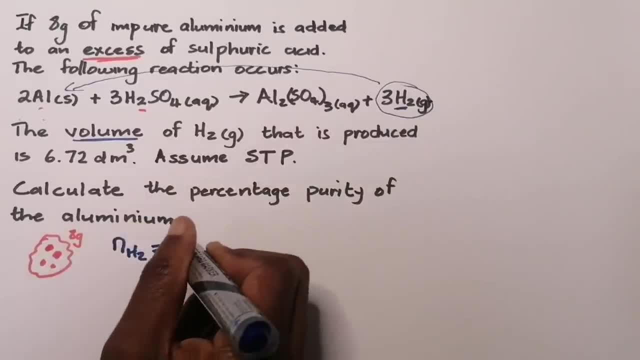 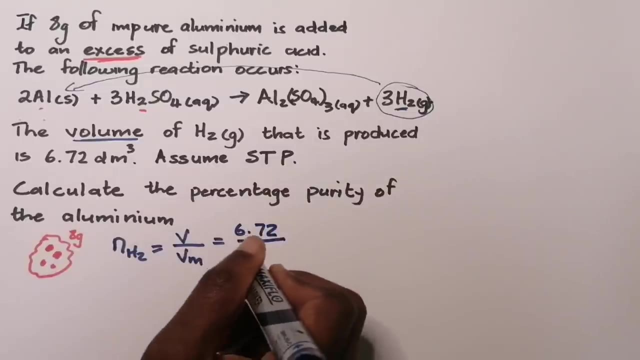 moles. these are the number of moles of hydrogen, right? so number of moles of hydrogen, that's going to be volume divided by the molar volume. so they gave us the volume. okay, they gave us the volume, it's 6.72. but we know that the molar volume at stp is 22.4 cubic decimeters per mole. okay, 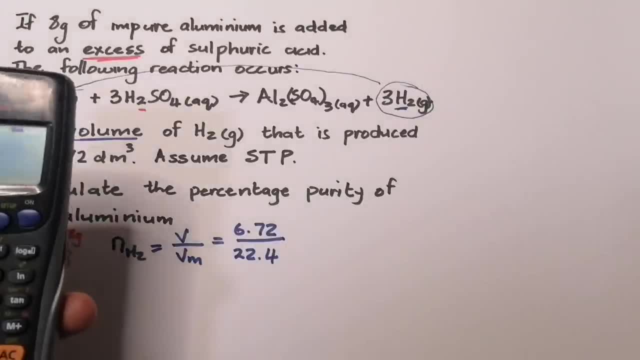 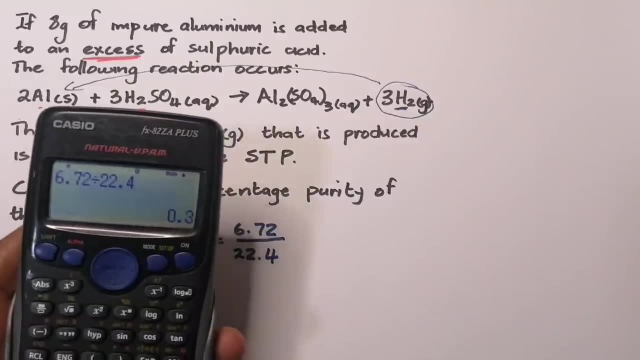 so now i'm going to say: all right, let's find out: sin 6.72, divide by 22.4. okay, that will give us 0.3 moles. okay, so it means that the number of moles of hydrogen that was produced is: 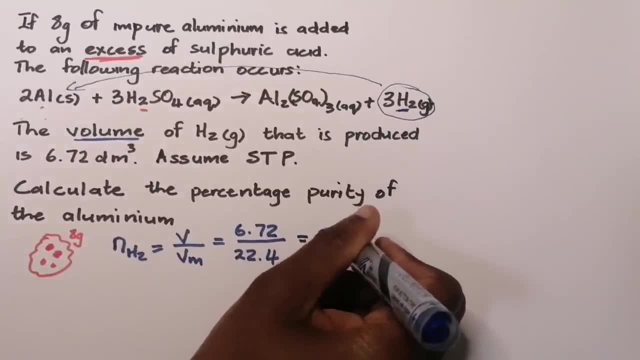 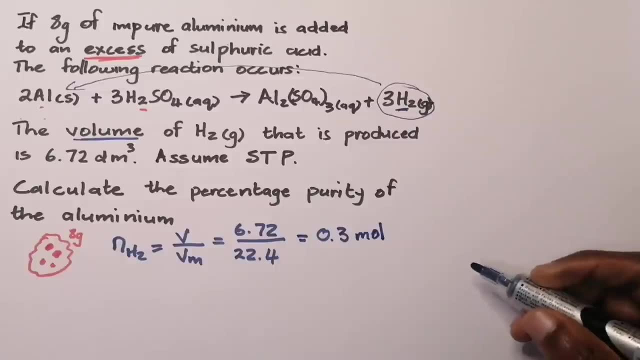 0.3 moles. okay, so that's 0.3 moles of hydrogen that we've got there right now. please, i want you to note, ladies and gents. then i'm going to say: okay, now that we've got the number of moles that we actually produced- remember, those number of moles were produced- 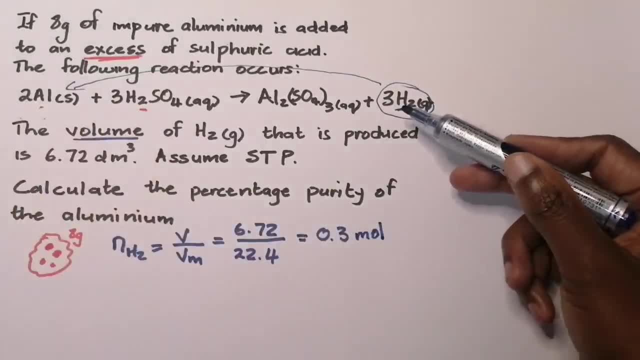 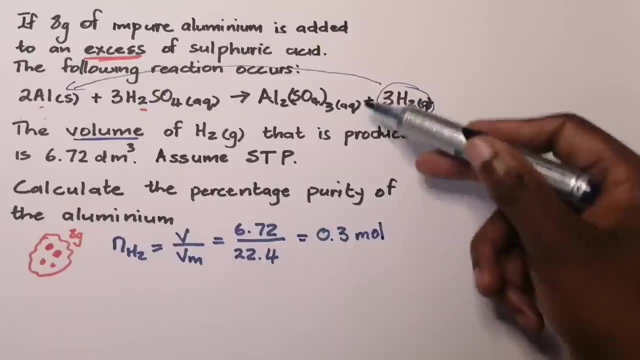 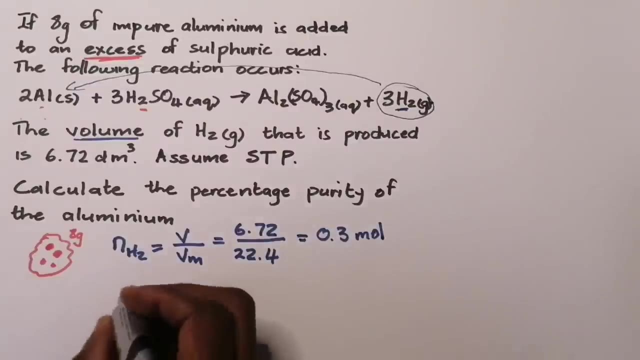 because of the bathroom rate. okay, so the the reaction with the sulfuric acid. okay, so i want to find out if i was able to produce this amount of hydrogen, then how much aluminium did i use? okay, so let's go to our mole ratios. okay, so it says for every two moles of aluminium. remember, we always start at. 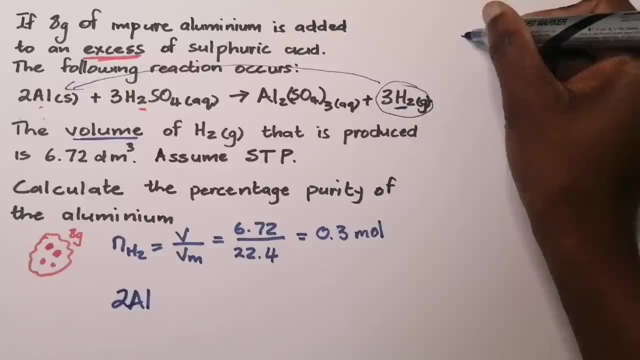 um, at our race with our ratios, rather. uh, if you don't mind, let me write over here. so i'm going to say, well, for every 2 moles of aluminium we always start at. at our ratio, with our ratios, rather, if you don't mind, let me write over here. so i'm going to say, well, for every 2 moles of aluminium, remember we. 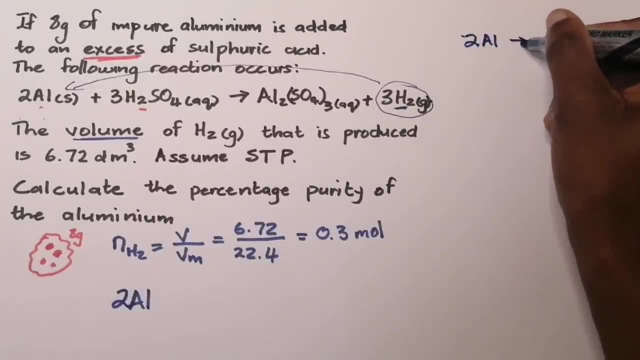 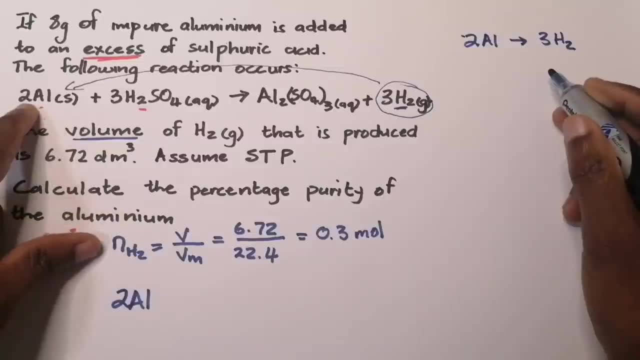 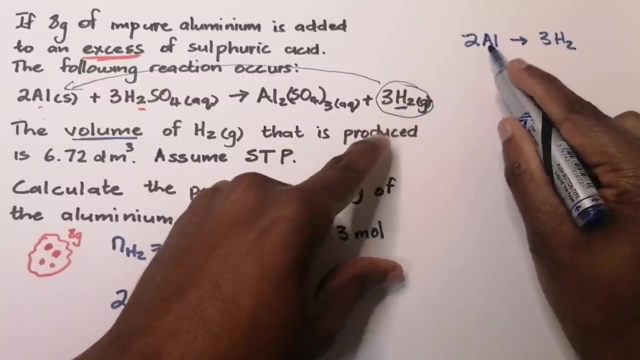 for every two moles of aluminium, i seem to produce three moles of hydrogen. okay, right, so i start with my ratios: two of aluminium produces three of hydrogen. why am i using aluminium and hydrogen? because i want to find out how much aluminium i get, okay, or i used rather in order to produce. 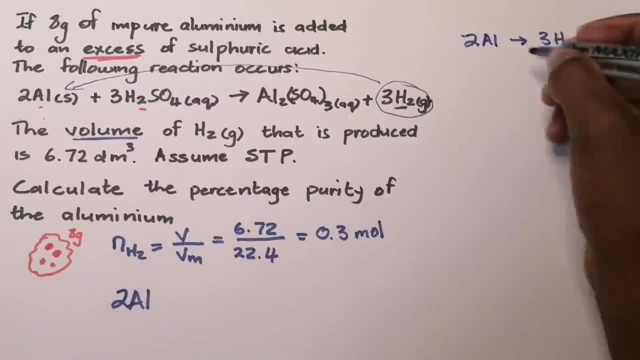 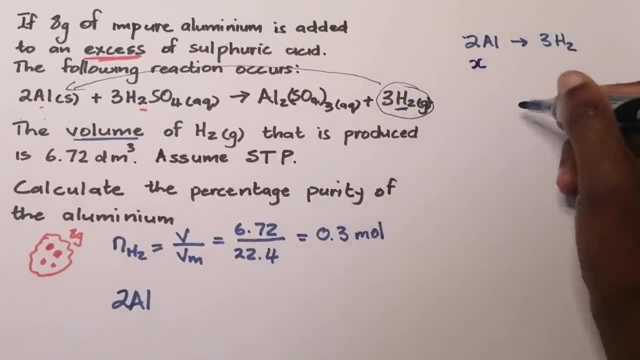 the hydrogen hydrogen. i've already gotten the number of moles, so now i'm going to say: for every two there's three. so therefore, for how much aluminium? i'm just going to use that as x. for how much aluminium am i going to produce 0.3 moles of hydrogen? okay, right, so you can cross multiply. 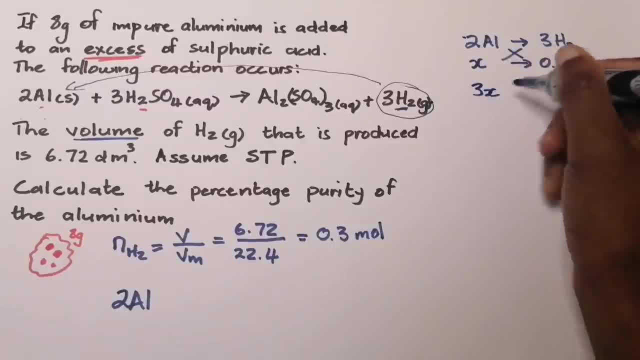 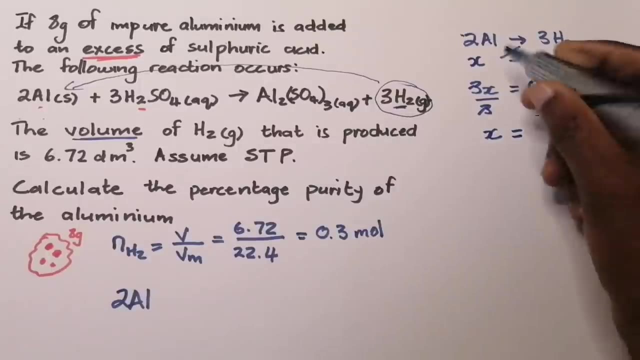 there, okay, so that's three times x. again, that's 3x 2 times 0.3. that's going to be 0.6, okay, and you can divide both sides by three there, of course, and so x. remember, what does x represent? in this case the number of moles of aluminium, right? so i seem. 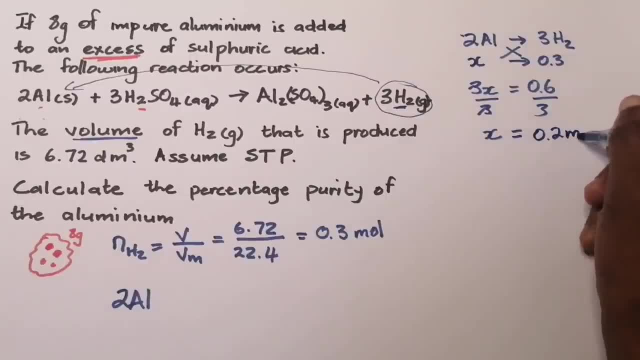 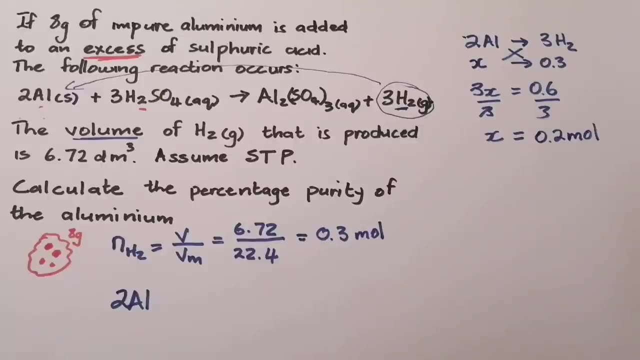 to get x to be 0.2 moles. so it means that the number of moles of aluminium was 0.2 moles. so it means that this is the amount of aluminium. okay, that actually reacted. okay, so of these eight grams, the actual amount, the pure amount of aluminium, was only 0.2 moles. now remember, you can't compare. 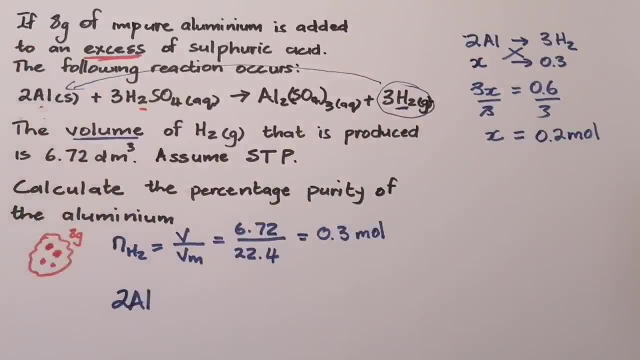 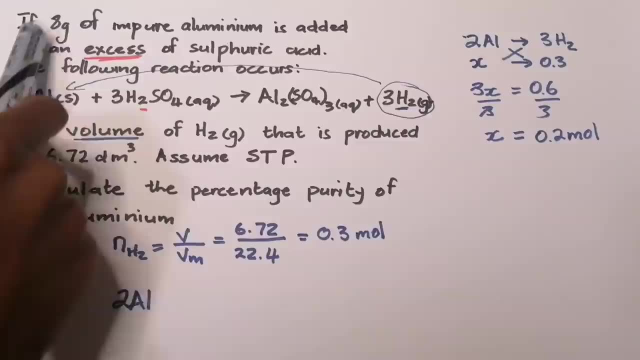 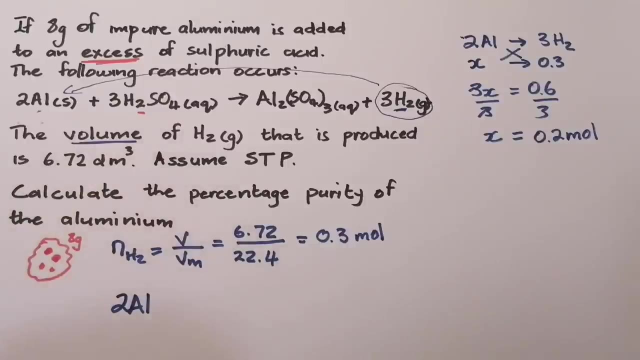 moles and grams. so what i'm going to do to calculate the percentage purity, let me find out. this is the total mess. all right, that mess that they gave me. that's a total mess, including the impurities. let me find out the mess of the actual aluminium. okay, so i'm going to say: 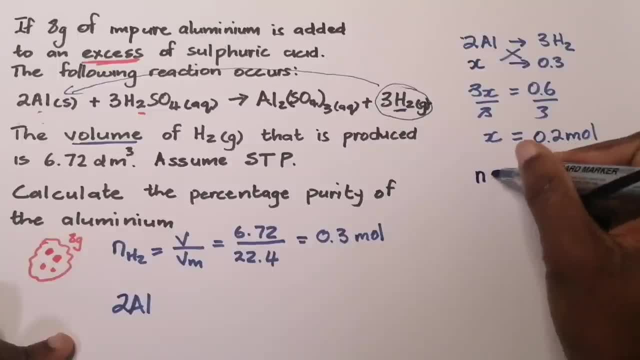 all right if i've got 0.2 moles. i'm- uh, the number of moles that's going to be mess divided by molar mess. what am i doing now? i'm trying to find out the number of moles of aluminium. okay, so i'm going. 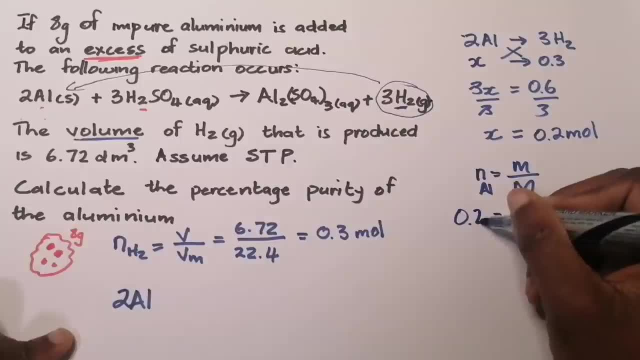 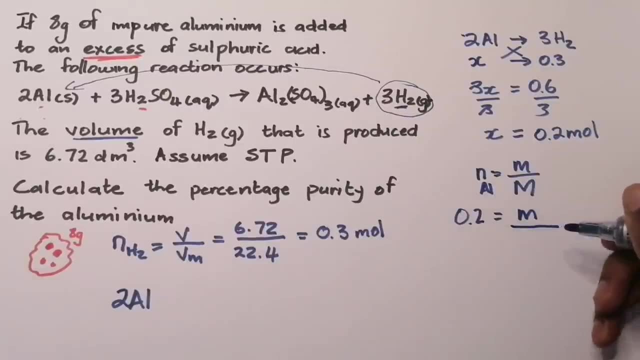 to say: okay, i know the number of moles, that's 0.2. i hope you're following, ladies and gents, right. so number of moles: that's mess divided by my molar mess. if you remember, we already had gotten that from the periodic table. okay, 10 rein the null part, that's 10. we could Searle that down to 30 exactly. 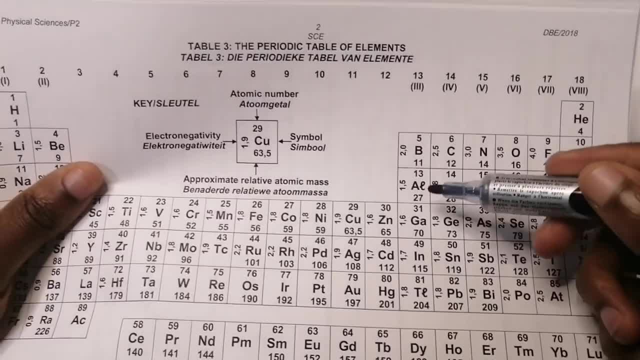 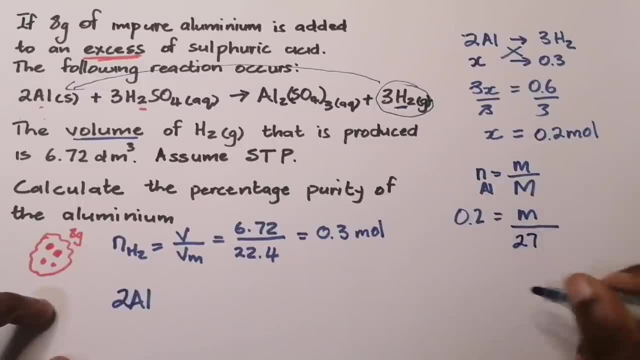 so, uh, aluminum, that will be 27 grams per mole, right, so that's the molar mass for aluminum. so that's 27 and all that. you simply do so, okay, 0.2, uh, multiplied by 27. okay, uh, i believe we will get uh 5.4. okay, so that's 27 multiplied by 0.2. okay, uh, that gives us 5.4 grams now. 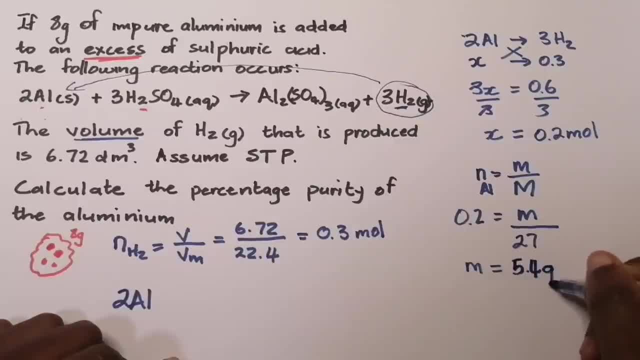 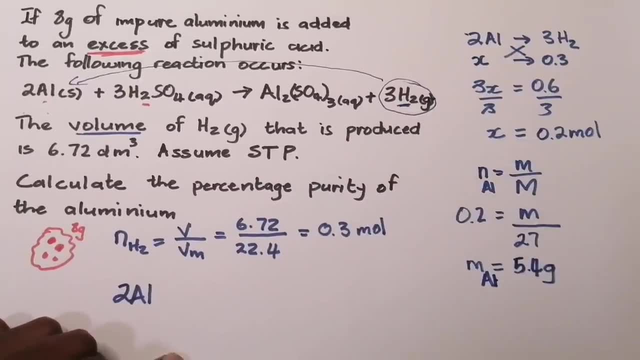 all right, now, ladies and gents, let's just find out what we've just done here. so this tells me of the eight grams that were given, all right, remember, that was impure. so of the eight grams, it was the aluminum, but it was also other impurities, other other substances, right, and remember, the other stuff did not react. 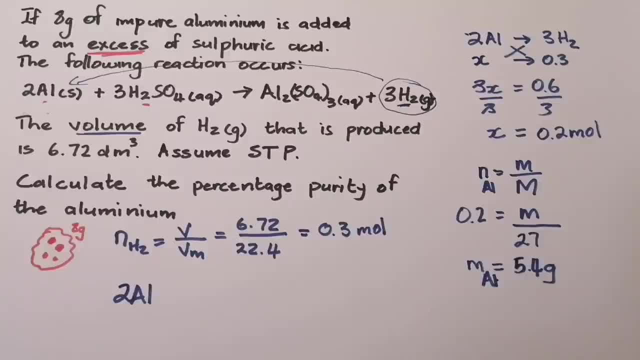 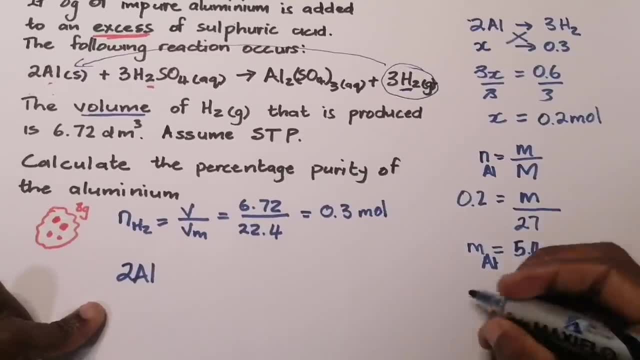 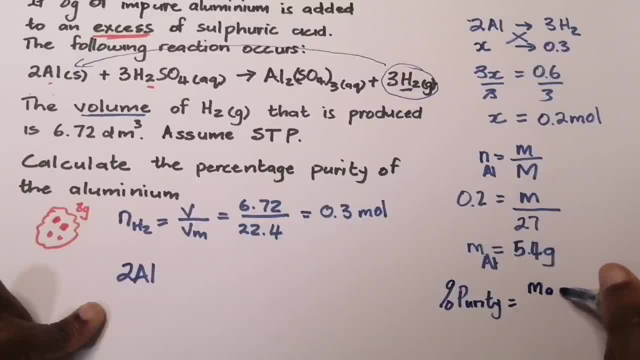 it's going to be the actual mass of aluminum divided by the total mass of what was given right, multiplied by um a hundred. so you can say it's the mass of the pure aluminum divided by the mass of the impure aluminum. okay, so that's. i just wanted you to get. it's the actual mass, all right, of the 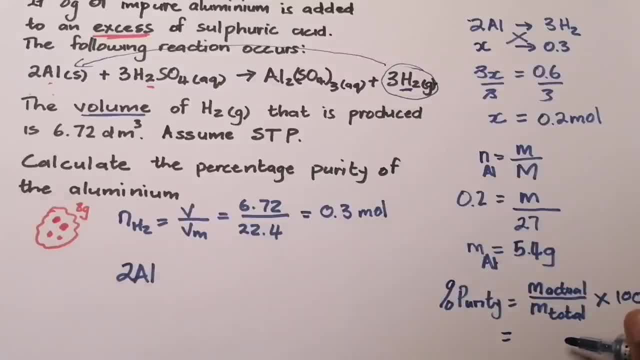 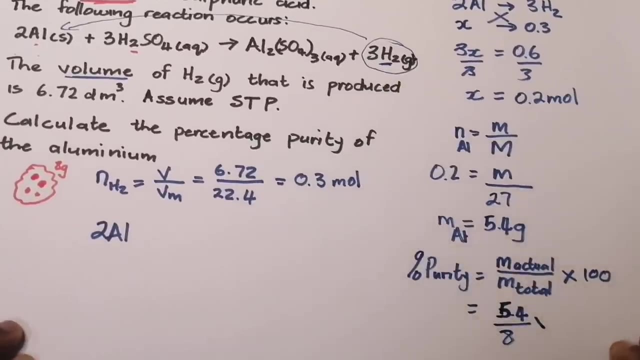 aluminum divided by the total or the mass of the impure sample, right? so in this case i'm going to have 5.4- okay, sorry about that- divided by 8, and okay, let's take that up a little bit. multiply that by a hundred, okay. 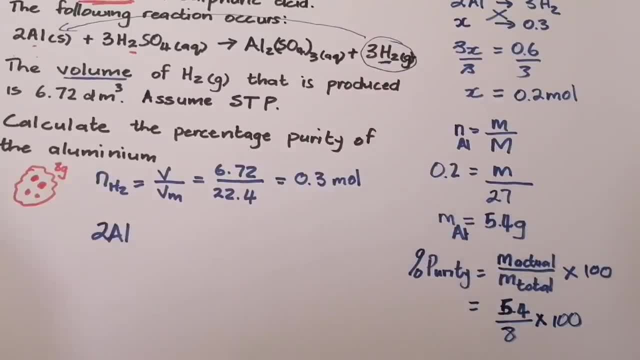 so, uh, what do you get? so that's 5.4 divide by 100, i mean divide by 8, okay, multiplied by 100 and you should get about 67.5 percent. okay, so that's 67.5 percent. so it means that sample there. 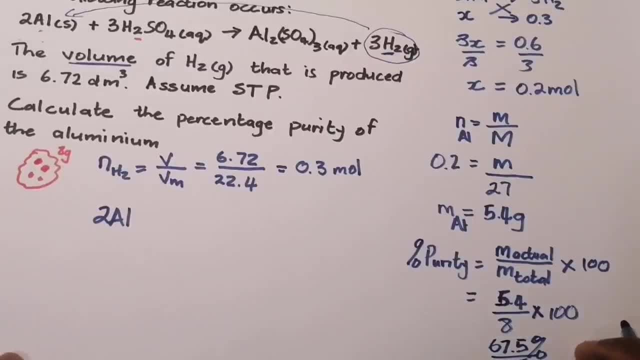 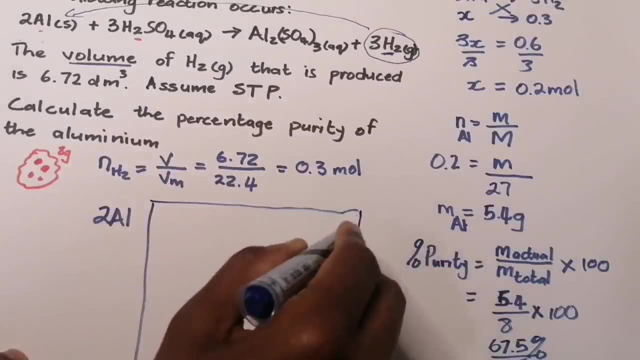 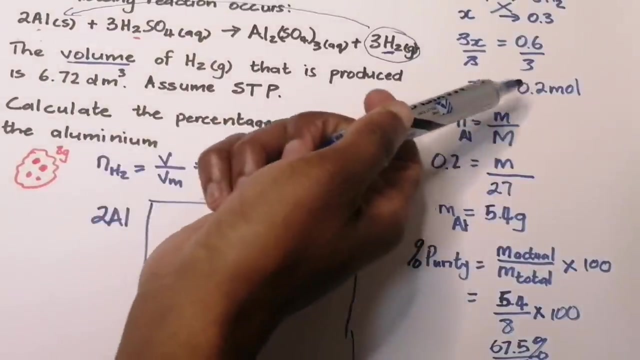 was actually 67.5 percent pure. now, for some of you, i'm sure you, you, you, you quite uh able to realize this by now. okay, there's nothing wrong. you could have actually used, uh, not the mass, or rather the number of mol, um, the, the number of mols, rather um. remember, here what we did was to convert the number of